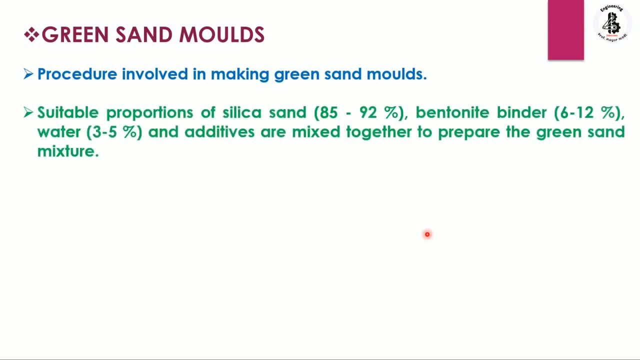 be having a proper mixture for making a green sand molds. it will be having a silica sand that will be around 85 to 92 percentage. used bentonite as a binder, which will be containing with a 6 to 12 percentage, with a water around 3 to 5 percentage, and additives are mixed together to prepare the. 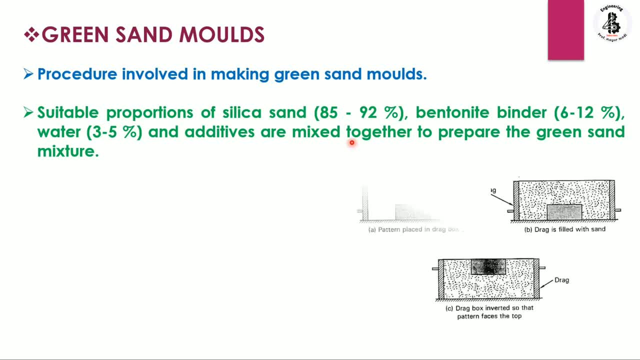 green sand mixer. so now, just you will see the different steps it will be to make a green sand mold. so for here the pattern which will be placed onto a flat surface with the drag box that will be enclosing it. so just you can see into this figure this is our flat surface and this rectangular box it will be considering as a 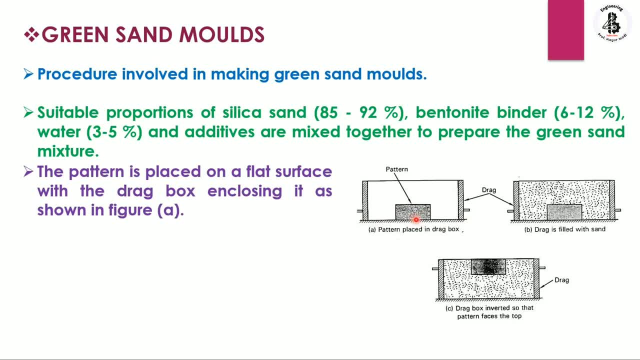 pattern. so now it will be resting onto that surface and this pattern now it will be enclosing by a drag. then after just you can see the parting sand that will be springed onto that, particularly to avoid for a green sand mixture that will be sticking onto that pattern. so that will be not. 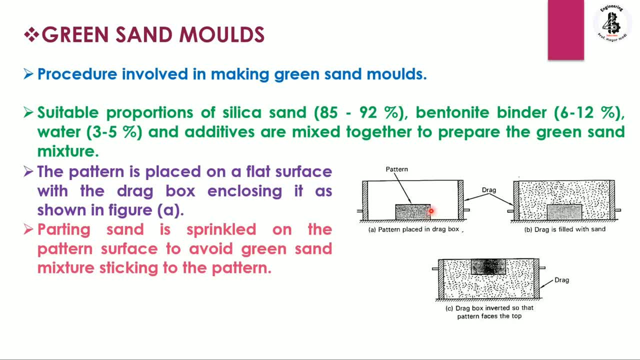 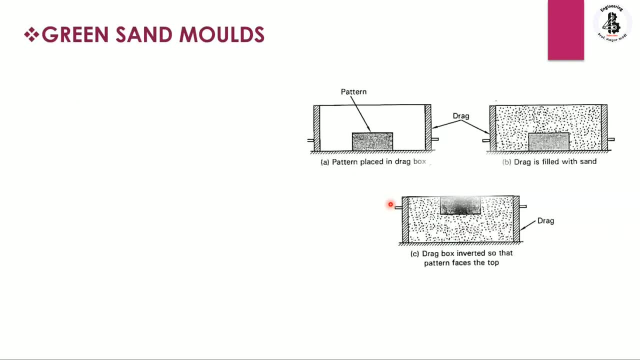 damaging the pattern as well as that will be not sticking with the patterns. now, after this sprinkling the parting sense, just you can see into the next steps, the drag box which will be filled with a green sand mixture and rammed manually till its top surface. just you can see all that. 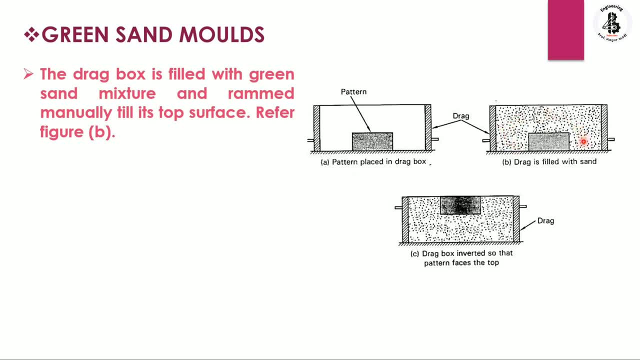 free space, or you can say into a drag box which will be filled by a green sand. then after the drag box, now it will be inverted. so what happens? the pattern faces at the top side. so just you can see into this figure c: by the inverting of this drag box, now pattern surface, it will be onto a top sides. 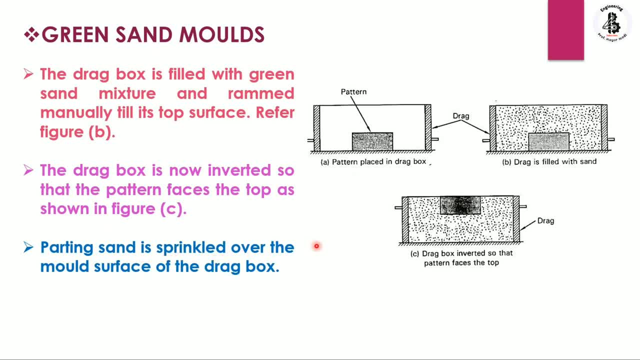 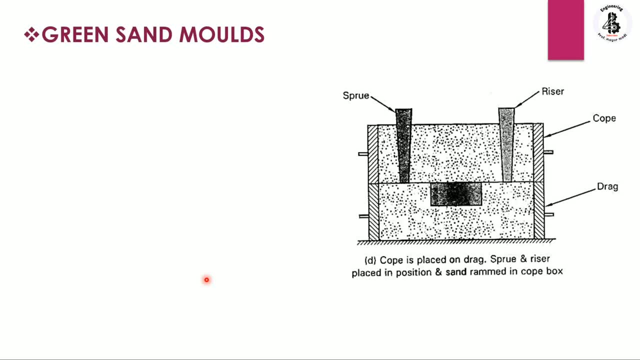 so what the parting sense will be like. so now you can see that the parting sense is sprinkled over a mold surface of the drag box. then after, in case of the green sand molds, just you can see the cop box is placed onto the top of. 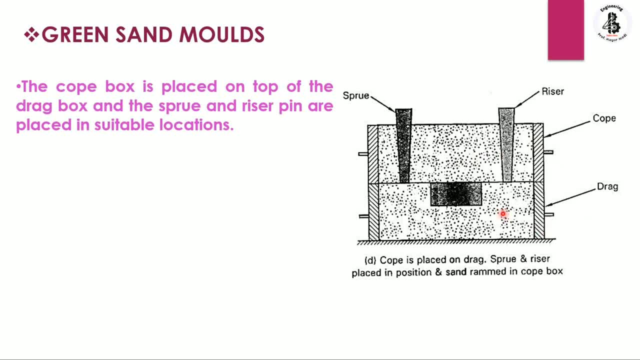 the drag box. so now into the bottom side. that will be the drag box. it will be filled with a green sand as well as with a pattern. now it will be covered by a cop, or you can see that cop and drag that will be separating by a parting line. so this one is our parting lines. so what? 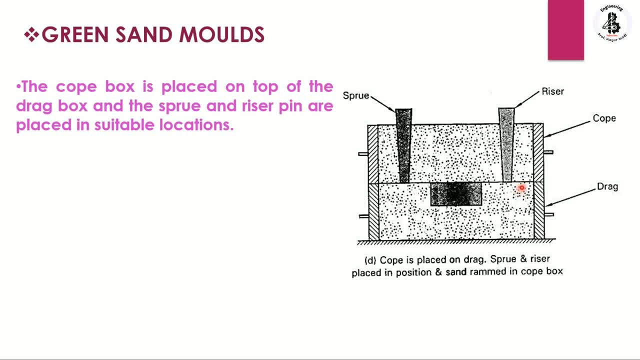 happens by the placing of the cop box onto the top of the drag box and the sprue and riser pin are placed at a suitable locations. so just you can see that will be our sprue mechanisms. so at the top side it will be the sprue basins, or you can say pouring basing, so the molten form of the metals. 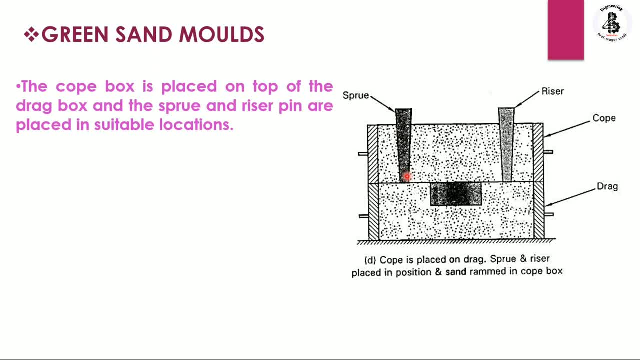 which will be pouring from the sprue and that will be the sprue basins. so that will be our sprue, will be having some getting component system design and fill with the cavity and that another side it will be the riser. but initially just you can make a passage for the sprue and a riser then 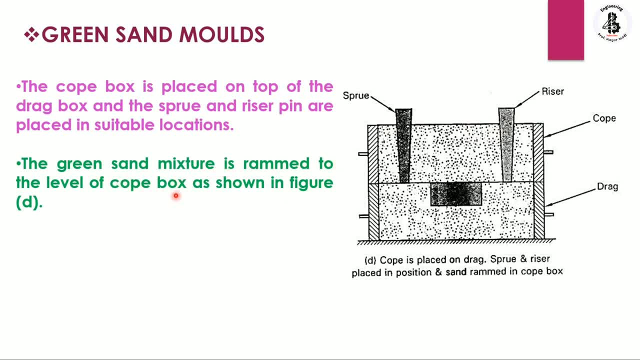 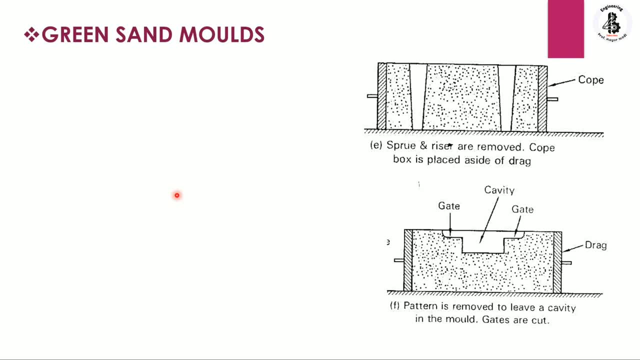 the green sand mixture is rammed to the level of the cop box. just you can see into the figure. then, after the next steps- and that will be, the sprue and the riser are removed from the mold, the cop box is lifted and placed aside and the 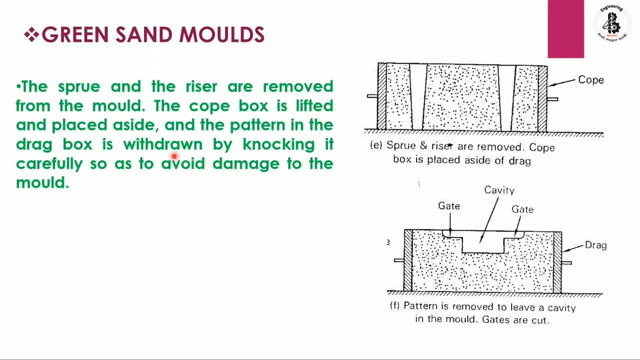 pattern is the drag box that will be withdrawing by the, knocking it carefully as to avoid the damage to the mold. so just you can see from this the pattern now it will be removing so it will be making a cavity. just you can see at both the side from that patterns it will be making the getting. 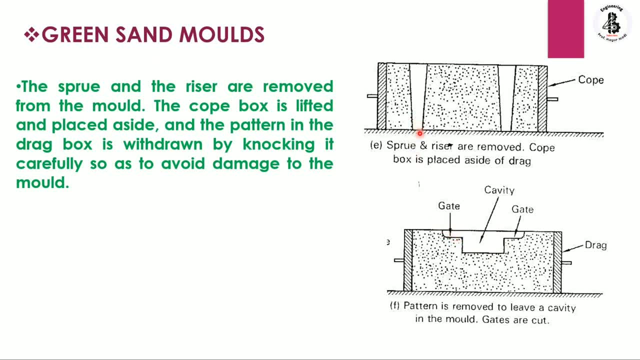 so this getting systems, it will be directly connected with these sprue systems and another side, that will be the another gate and it will be connected with a riser. so the gates are cut using the hand tools to provide the passage for the flow of a molten metal. 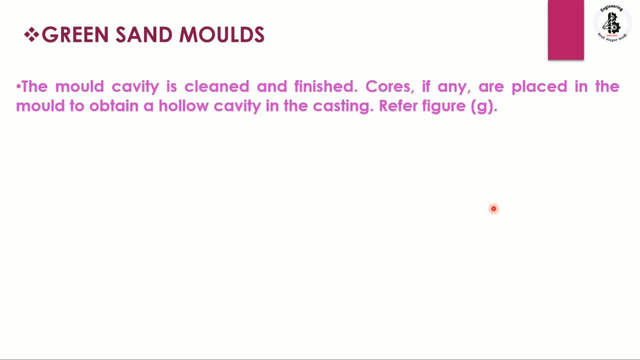 then after, in case of the green sand, the mold cavity is clean and finished. so the core is being used, so the cores, if required, so that will be placing into the mold cavity, if there will be the requirement of the hollow castings, so the core is being used. 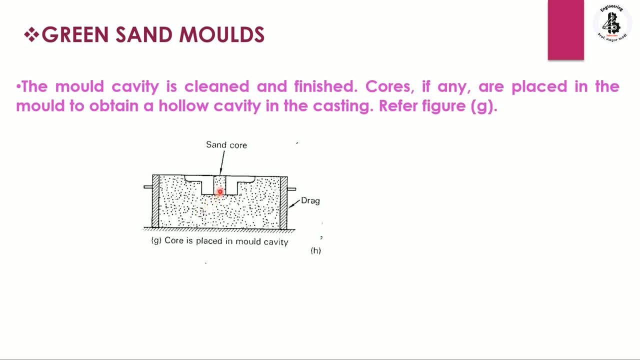 so just you can see into the figure we are making a hollow castings. so this core which will be placed into the mold cavity, so that would be also considering as a vertical core, so that would be easily placing into the mold cavity. so as from the complexity of the shape and size it will be. 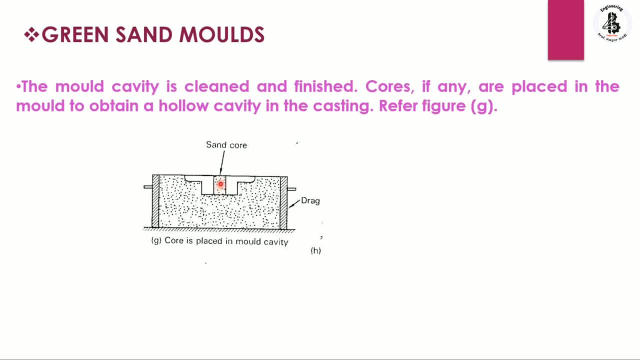 utilization of the different cores. so here that will be the vertical. you should also use a horizontal, then key score, then hanging course, as per my requirements. now that will be the cop that being placed onto the drag and vent holes that will be also made for escaping the hot gases. 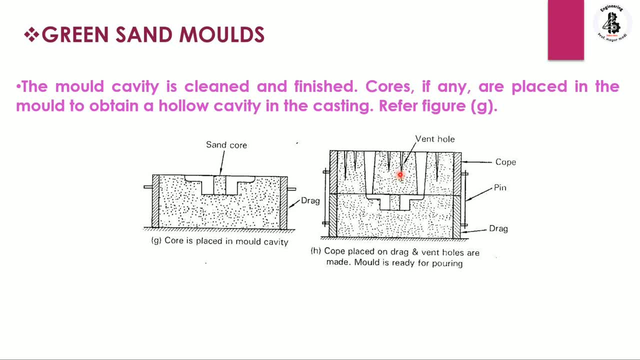 during the pouring of the molten form of the metal. so now, just you can see, this is our drag portion which will be connected with the help of pin, with a cope, and here that will be the sprue and another side that will be the riser. so molten form of the metal which will be fill. 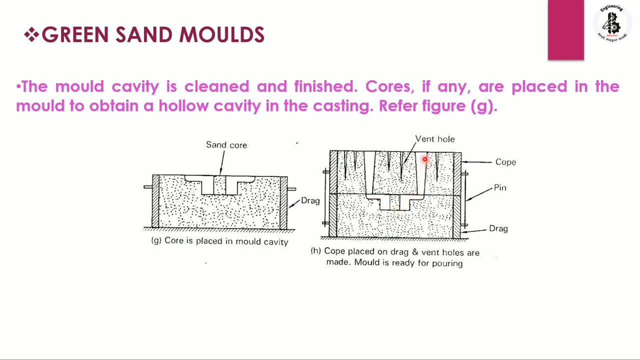 into the mold cavity and through the riser you can ensuring that the hundred percent filling of the mold cavity. so now, the cope is now placed onto the drag box and both are aligned with the help of the pins. some vent holes are made to allow the free escape of the gases from the 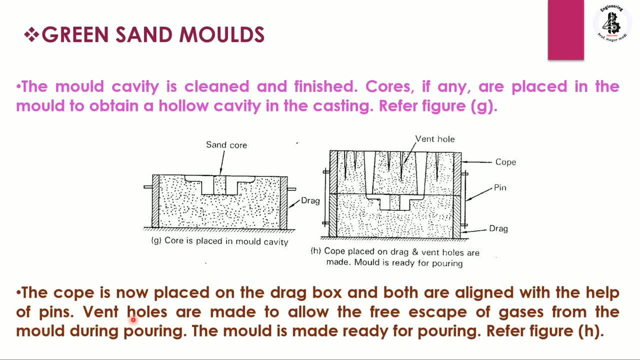 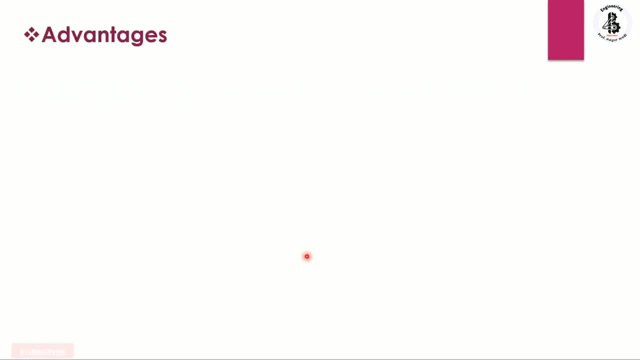 mold during the molten metal is being pouring. so the mold is made ready for pouring. just you can see into last figure then. for this there is some advantages, like green sand molding is adaptable to machine molding. then, second, there is less mold distortion than in any dry sand molding process. then time and cost associated. 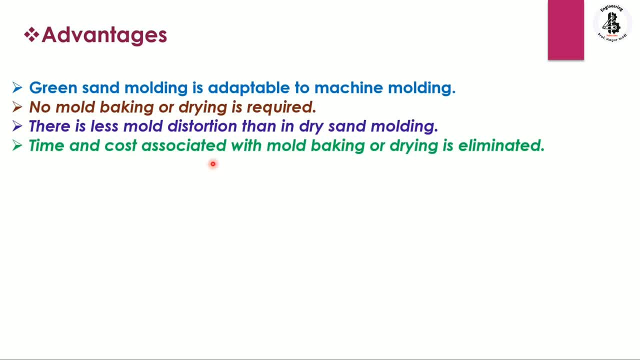 with mold backing, or you can say drying is eliminated, then more thing like green sand molds: having a smaller depth permits the escape of the mold gases. that will be without any difficulties in green sand moldings. flasks are ready for re-painting or re-painting, so you can see that.